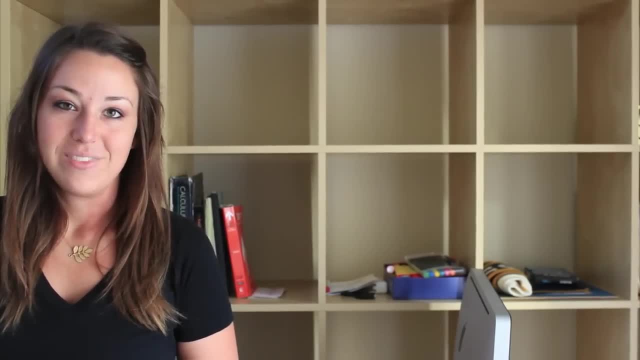 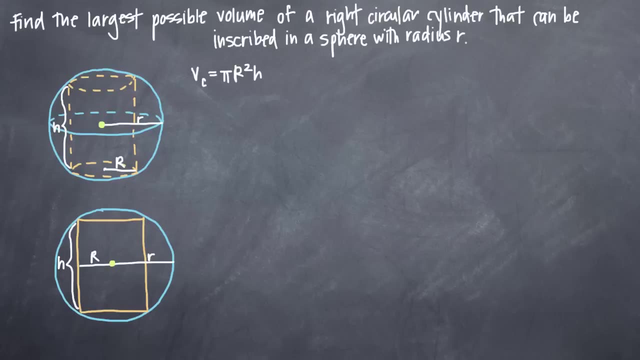 derivative of the optimization equation to find the volume. Let's take a look In this particular problem. we've been asked to find the largest possible volume of a right circular cylinder that can be inscribed in a sphere with radius r. So, as with any optimization, 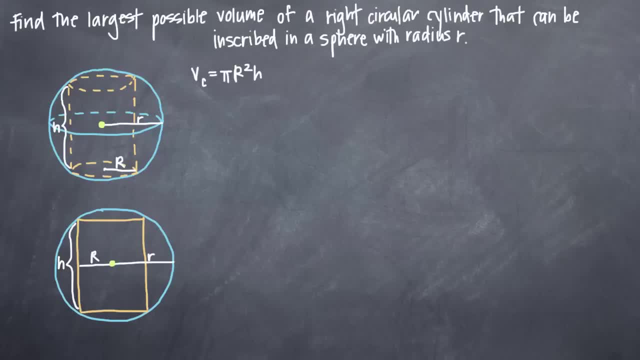 problem. the first thing we want to do is draw a picture of what we know. So we've been told that we're inscribing a cylinder into a sphere. That means that we're trying to fit a cylinder inside of a sphere. So I've drawn the sphere here in blue and I've drawn 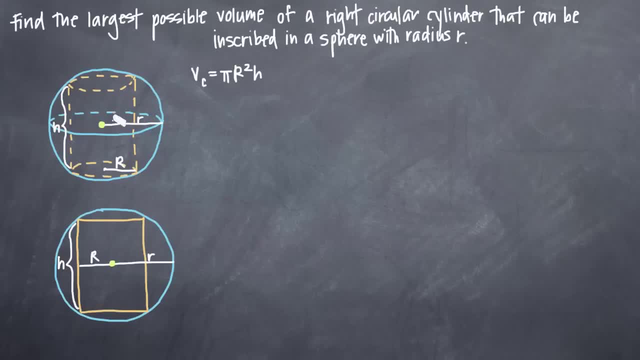 the cylinder in orange. We also want to label every part of this diagram that we can. So we know that the radius of the sphere has to be equal to the radius of the cylinder, So we've gone ahead and labeled the radius of the sphere as r. We also know that, since 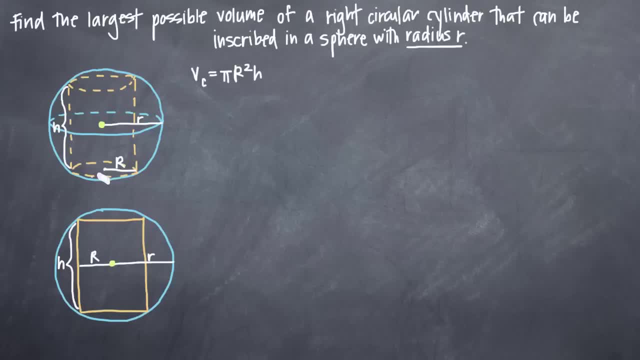 this is a right circular cylinder, that we're going to have a radius of the cylinder, so we can go ahead and call that capital R and we've labeled that as well. And then, finally, the other thing we know at this point is that the cylinder is going to have a height, Obviously. 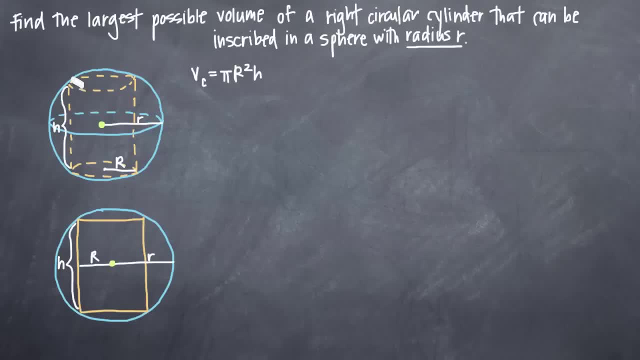 we don't know what it is yet, but we know that it's going to have a height and we can call the height r. So we've labeled the radius of the cylinder as r. So we've labeled the radius of the cylinder as h. So we've drawn a picture of that and then we've also gone. 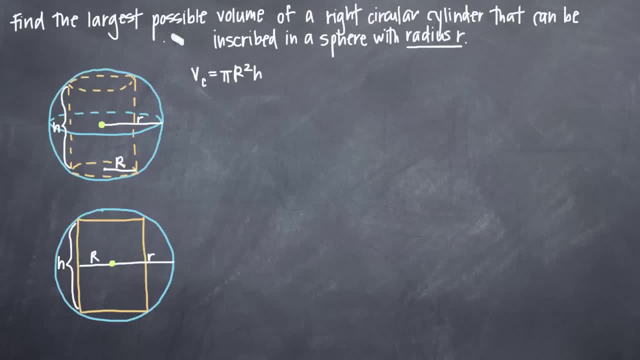 ahead and written down the formula for the volume of the cylinder. We know that we're going to have to find the largest possible volume of the right cylinder. so we can say that the volume of the cylinder v sub c is equal to pi. capital, R squared h: Capital. 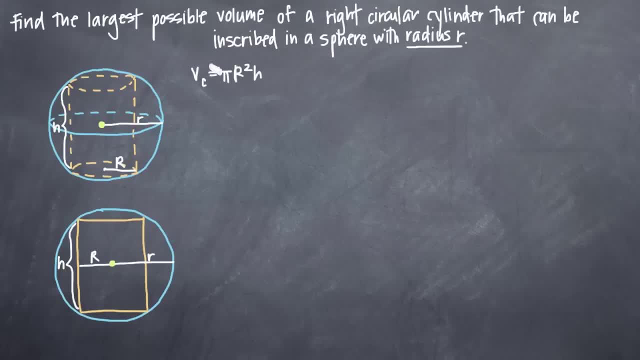 R squared, because we're talking about the volume of the cylinder and we've indicated that the radius of the cylinder is capital R. So now that we've drawn a picture of the cylinder, we know that the volume of the cylinder is capital R squared h. So now that we've 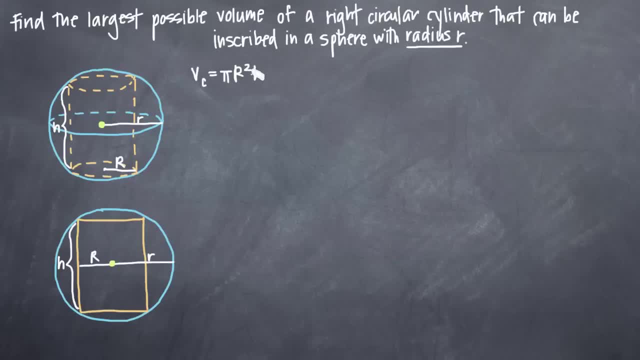 identified the volume of the cylinder. we can go ahead and write down what we know. We need to identify optimization and constraint equations. Remember that the optimization equation will be the equation that we're trying to optimize, meaning the equation that we're trying to minimize or maximize, Since we were asked to find the largest possible volume. 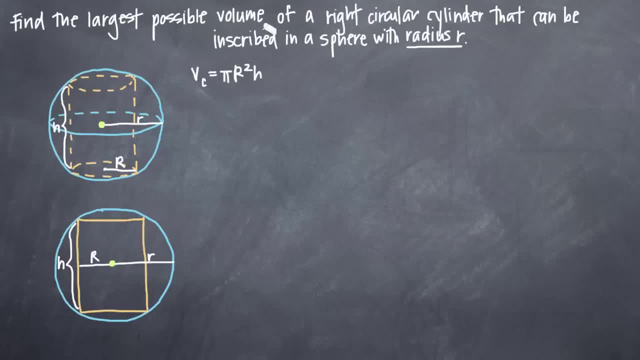 that means our optimization equation has to be an equation for volume, So this volume equation we have here for the volume of the cylinder will be our optimization equation. We also, though, need a constraint equation, and the constraint equation is the equation that limits us, So we're trying to maximize the volume as much as we can within the constraint. 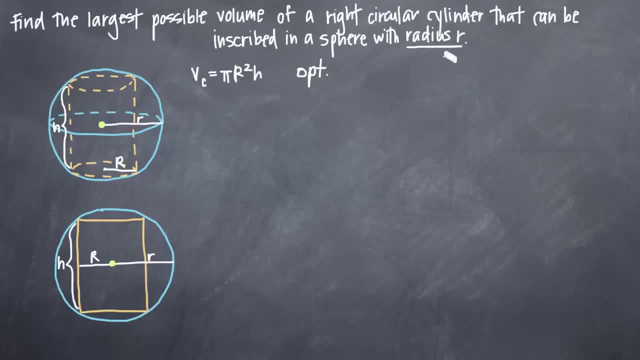 that the radius of the sphere must be R. That's the only condition that we've been given, the only constraint within which we have to work. So we know that the constraint equation has to be an equation involving R, and keep in mind that this is lowercase r, or the radius. 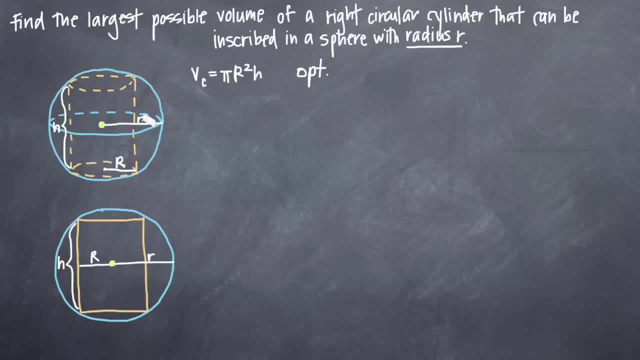 of the sphere. As it turns out, we don't have to write down the volume of the cylinder, we just have to write down the radius of the cylinder. We don't have an equation yet that involves lowercase r or the radius of the sphere, so we need to find one. More specifically, we need to. 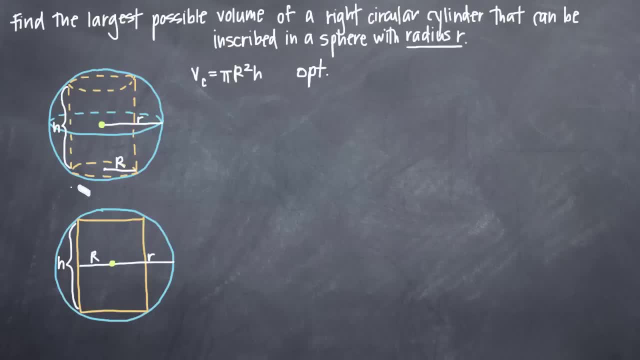 find an equation for the radius, that is, in terms of capital R, the radius of the cylinder and H, so that we can relate lowercase r, capital R and H. So the way that we're going to do that is by imagining that we take a cross section of the sphere that we've diagrammed. 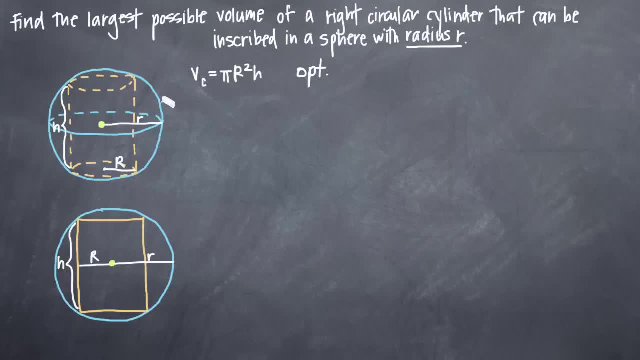 up here. So if you can imagine, if we cut out a slice of this sphere vertically and we had a vertical slice like this, we'd have the height H here, we'd have the radius of the sphere diagrammed here with lowercase r and we'd have the radius of the cylinder. 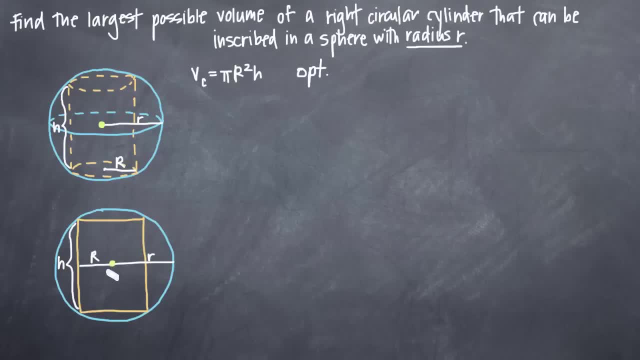 diagrammed here with capital R. The key to relating these three variables is realizing that the radius of the sphere is R everywhere. So not only do we have the radius of the sphere equal to R here, but obviously from the center of the circle to this point here the radius is also R. So the reason that this is so great is because we're going to be able to write down the radius of this sphere as well, and that the radius of the sphere has to be equal to R, and that this is what we're actually going to be able to write down. 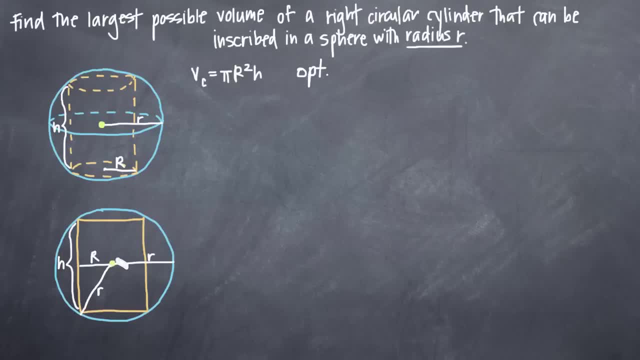 What I found great is because once we realize that this length from the center of the sphere and the cylinder to the corner of the cylinder or the edge of the sphere is R, we realize that we have a right triangle And we know that we can relate the three sides of the 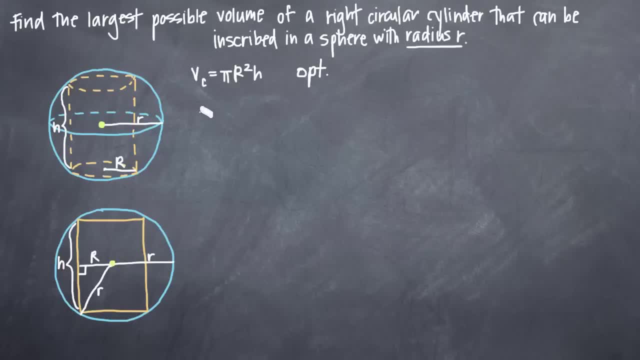 right triangle with the Pythagorean theorem. Remember that the Pythagorean theorem is just a squared plus b squared equals c squared, Where a squared and b squared are two sides of the triangle, c squared being the right side. So that's the Pythagorean theorem and plus c squared equals a squared And that's the 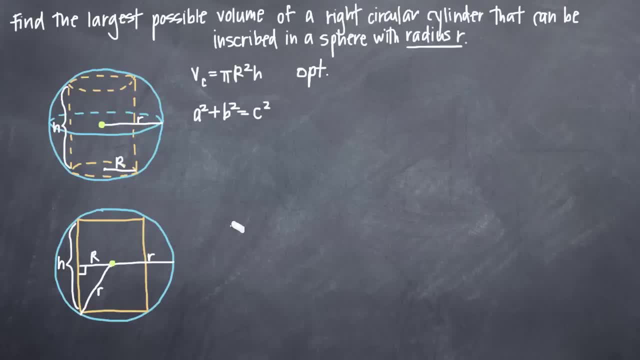 the hypotenuse of the triangle. We already know that the hypotenuse of the triangle is lower case r, or the radius of the sphere. so we can say that this is a squared plus b squared, equals r squared, and now we just need to plug in the other two sides. We know that one of 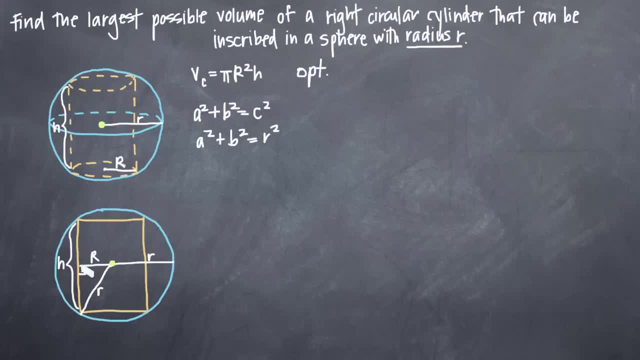 the sides is capital R. We know that the other side is actually h over 2, because the height of this rectangle here is h, but the height of this portion right here is just h over 2.. So we'll plug in h over 2 for a and square it. We'll plug in r for b and square that. 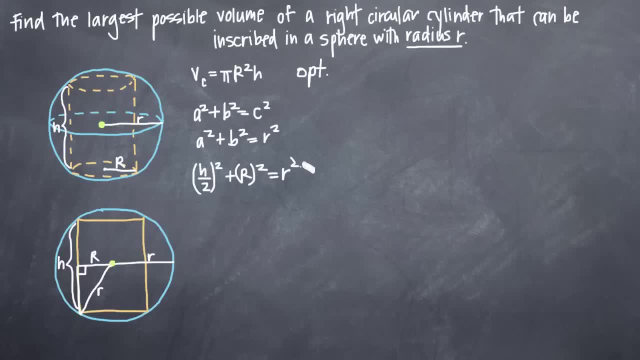 and then we already know that that's equal to the hypotenuse lower case r and that's squared. So now we have an equation that relates lower case r, capital R and h, and this is our constraint. Subtitles by the Amaraorg community. 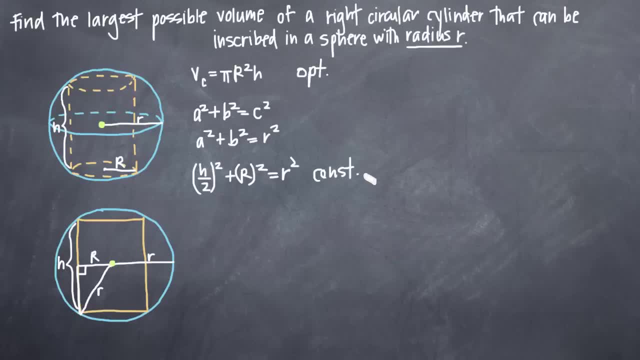 equation because, remember, our constraint equation had to involve lower case r. Now, once you have a constraint equation and an optimization equation, your goal will be to solve the constraint equation for one of the variables in your optimization equation so that you can make a substitution. You need to get your optimization equation in terms. 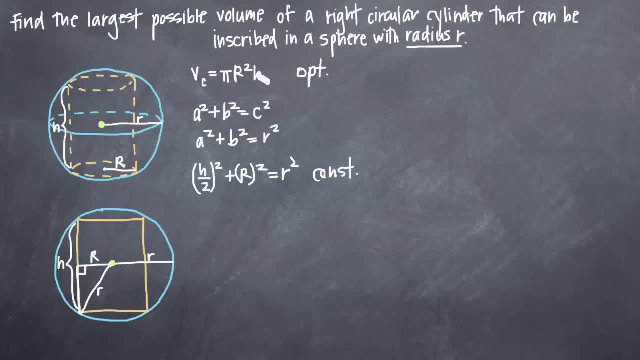 of one variable only. Right now, we have two variables involved in our optimization equation- capital, R and h- So we need to eliminate one of them, and the way that we're going to do that is by solving the constraint equation for one and making a substitution. 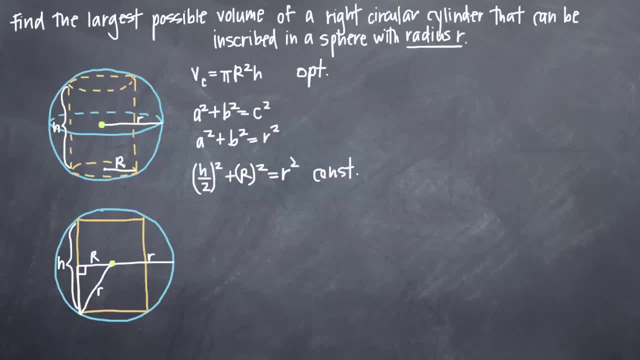 So let's go ahead and solve for r squared. As you can see, we have r squared right here and we also have r squared up here. So if we solve for r squared in our constraint equation, we can make a really easy substitution, as opposed to having to solve for h, which may. 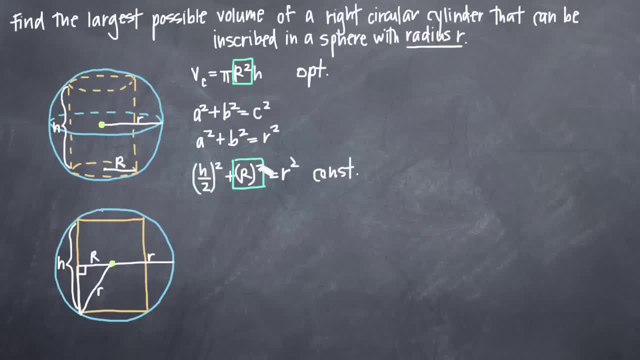 be a little bit more difficult. So let's go ahead and solve for capital R squared The. The way that we'll do that is by taking the square of h over 2, and we'll get h squared over 4, plus capital R squared is equal to lowercase r squared. 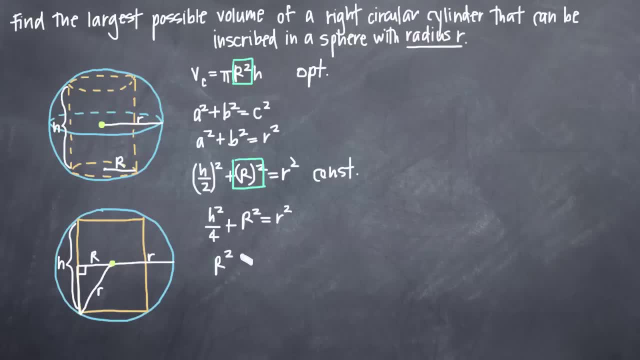 When we subtract h squared over 4 from both sides, we'll get capital R squared equals lowercase r squared minus h squared over 4.. So now we've solved for r squared and we can go ahead and plug the whole right side here in for r squared up in our volume equation. 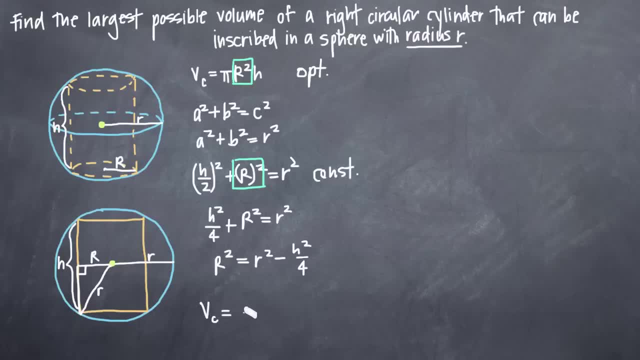 When we do that we'll get. the volume for the cylinder is equal to pi times. here's where we're plugging in: r squared minus h squared over 4, all multiplied by h. Now our volume equation, or our optimization equation, is in terms of one variable only. 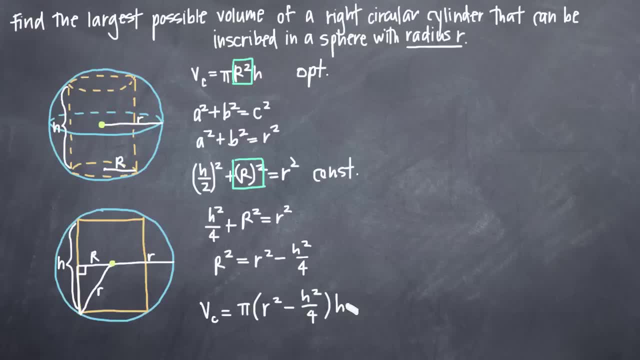 You might think it's in terms of two variables, because you see lowercase r and h. However, remember that lowercase r is equal to r squared minus h, squared over 4, plus capital R, squared over 4, plus capital R squared over 4 times h squared over 4 times h squared. 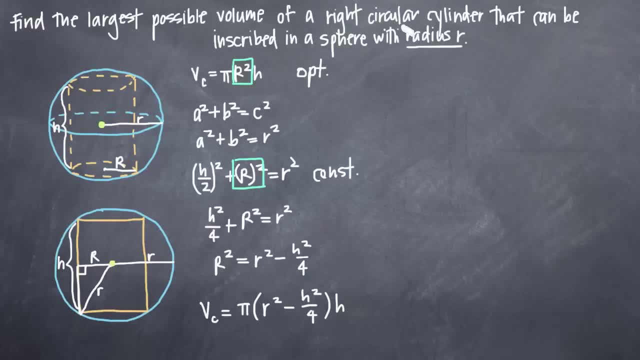 over 4 times h squared over 2.. Number 2. We're just going to take the volume of the cylinder and we're going to give it a constant, because we've already seen that the lowercase r is actually a constant, because it's the 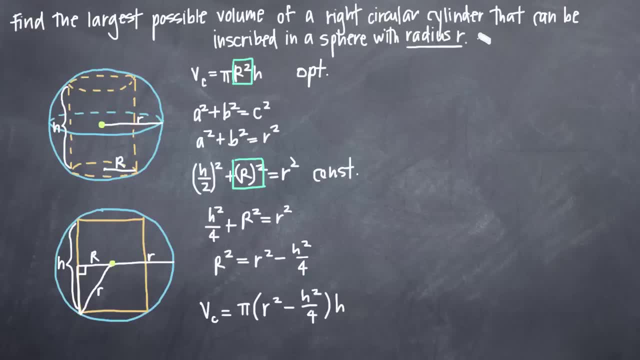 radius of the sphere, which is never changing, and we've been asked to find the largest possible volume of the cylinder inscribed in the sphere with radius r. They could have just as easily asked us to find the largest possible volume for the cylinder inscribed in a sphere with radius 4.. 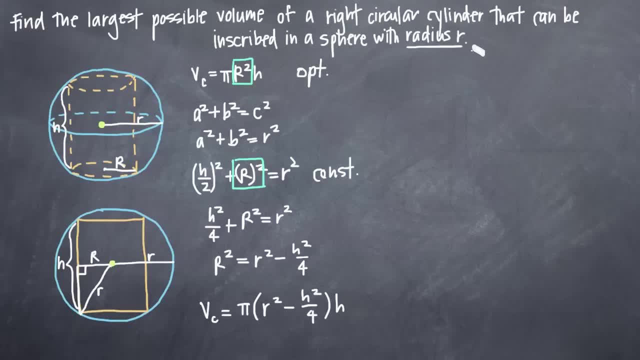 If they had done that, r obviously would be a constant, it would be 4.. In this case it represents exactly the same thing. We're going to treat it as a constant, and so that means that our volume equation here only has one variable, and that's 8.. 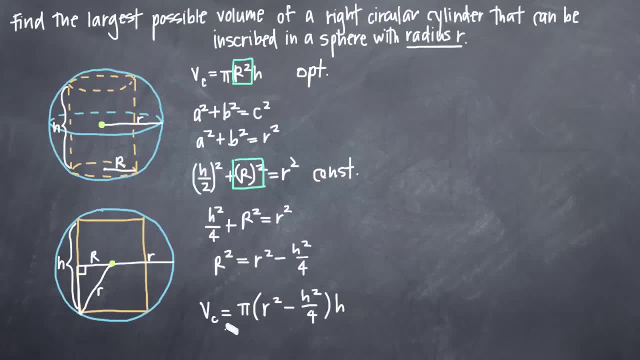 So now that we have our volume equation or our optimization equation, in terms of one variable only, our next step will be to simplify as much as possible and then find the derivative of the volume equation. So let's go ahead and simplify. first, We're going to multiply each term inside here: r squared minus h squared over 4, by both. 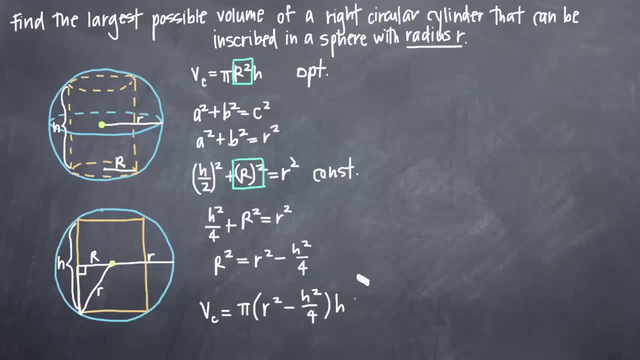 pi and h to simplify. So we'll get: the volume of the cylinder is equal to. we have pi times r squared times h, so we'll get pi? r squared h. and then we have pi times negative h squared over 4 times h, so we'll get minus pi over 4 h cubed. 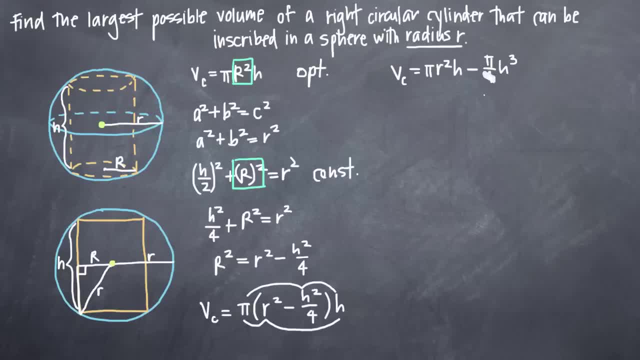 So that's as simple as we can get our volume equation. so now we're going to go ahead and take the derivative of the volume equation and then set it equal to 0. So the derivative we can call the derivative of v with respect to h or dv over dh. 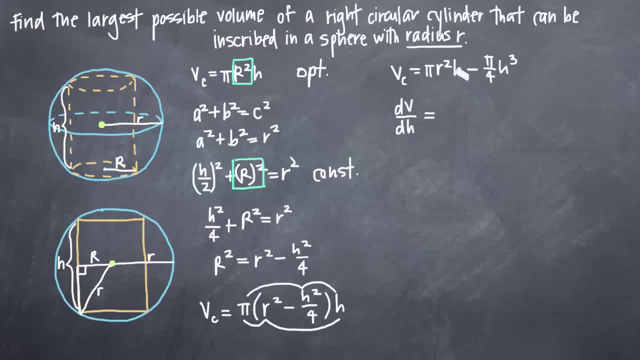 We're going to take the derivative of the right-hand side with respect to h, keeping in mind that r is a constant. So if we take the derivative of the first term, pi r squared h, remembering that r squared is a constant, the derivative is just pi r squared. 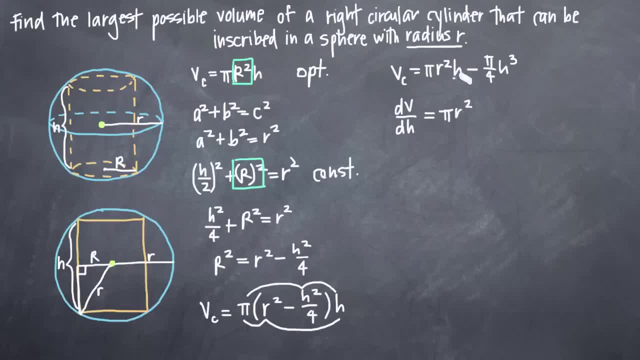 So we can multiply that by pi r squared h and we'll give it a derivative of pi r squared h plus the derivative of pi r squared h, because this is the same here, if h is our variable as taking the coefficient, here pi r squared. 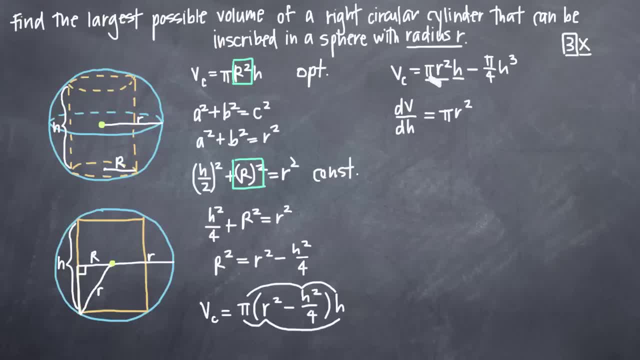 It's the same thing as taking the derivative of 3x, for example, where x is the variable and 3 is the constant coefficient: Pi r squared h. since r is a constant, that whole thing is the constant coefficient. So the derivative of pi r squared h is just pi r squared. 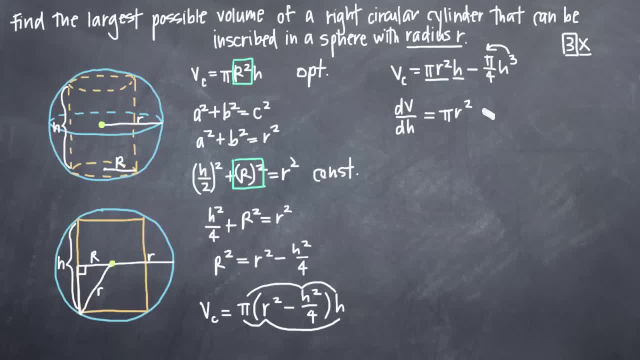 one from the exponent. so we'll get minus three pi over four h squared. So now that we've got our derivative, we want to go ahead and set it equal to zero and solve for h. So in order to solve for h, let's go ahead and add three pi over four h squared to both. 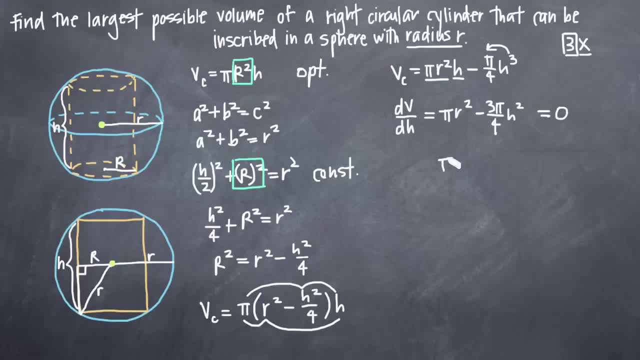 sides, We'll get: pi r squared is equal to three pi over four h squared. Let's go ahead and multiply both sides by four. We'll get four pi r squared is equal to three pi h squared. And now we can go ahead and divide both sides by three pi. 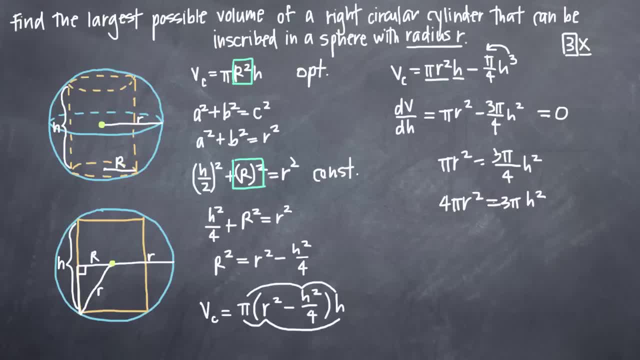 When we do that, the pi's will cancel and we'll just be left with four. r squared divided by three is equal to h squared, So now we have our derivative To solve for h, we'll take the square root of both sides, and when we take the square, 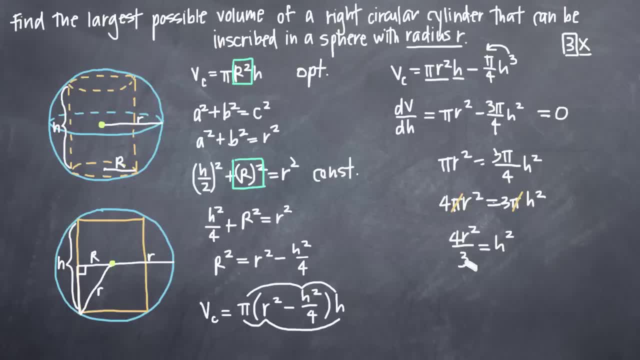 root of both sides. we can take the square root of the numerator and the denominator of the left-hand side separately. So the square root of four r squared is just two r and the square root of three we'll go ahead and leave as the square root of three and that will be equal to h. 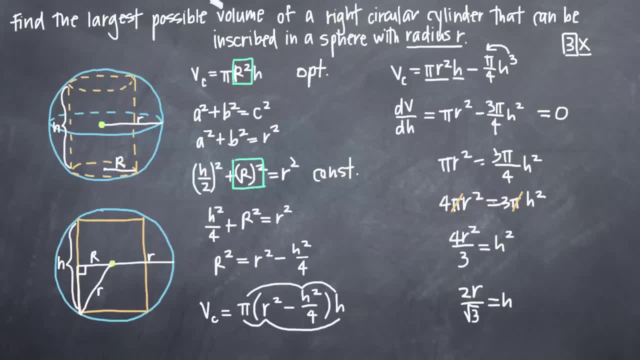 Now that we have a value for h, we just need to return to our original problem and remember what we were actually asked to find. Remember that we need to find the original problem. Remember that we were asked to find the largest possible volume of the cylinder. 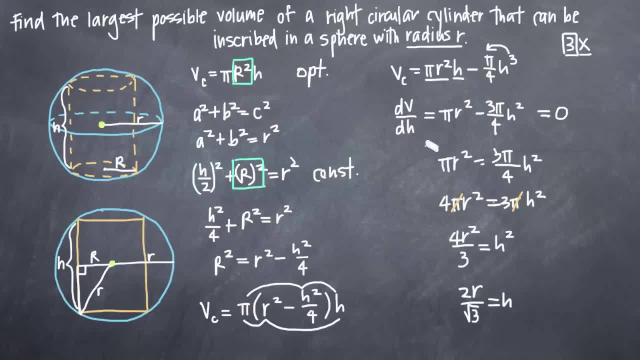 So we need to go ahead and plug in our value for h into our volume equation. This was the last good volume equation that we had, so let's go ahead and plug two r over the square root of three into this volume equation for h. 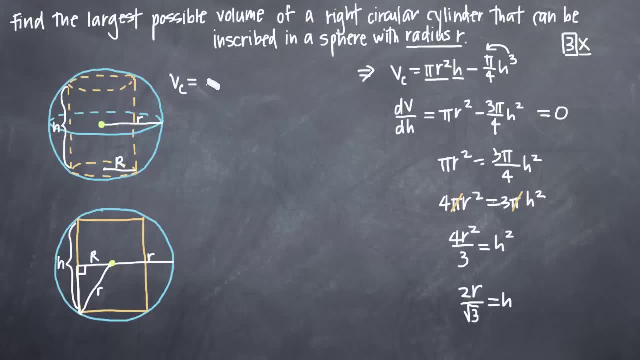 When we do that we'll get. the volume of the cylinder is equal to pi r squared times two r over the square root of three, minus pi over four times two r over the square root of three cubed. Now that we've plugged in h, our next step is just to simplify the volume equation as: 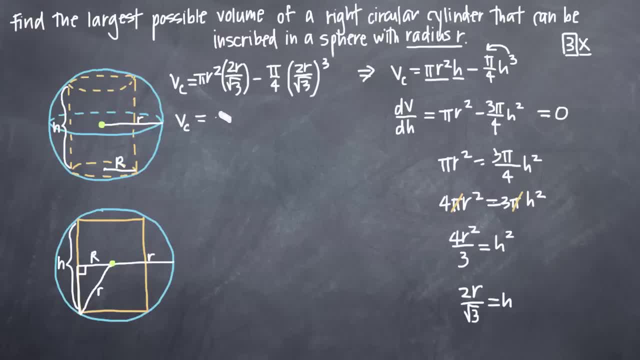 much as possible. So we get that the volume of the cylinder is equal to two pi r cubed divided by the square root of three. So that's equal to pi over four times two r over the square root of three, minus pi over four. 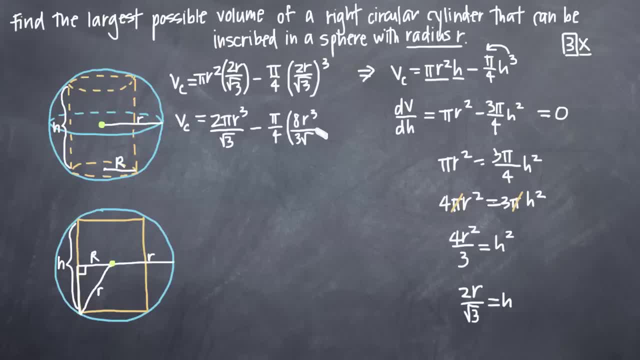 When we cube two r over the square root of three, we get eight r cubed divided by three root three. When we distribute the pi over four across the eight r cubed over three root three, we'll get And the eight will become a two. 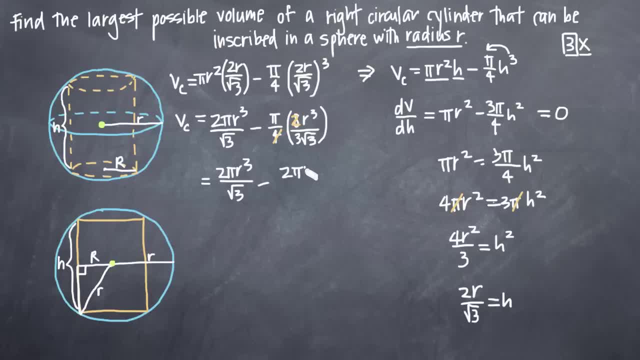 And so what we get is two pi r cubed divided by three root three. Now, in order to find a common denominator, all we need to do is multiply this first term here by three over three. So we get six pi r cubed minus two pi r cubed. 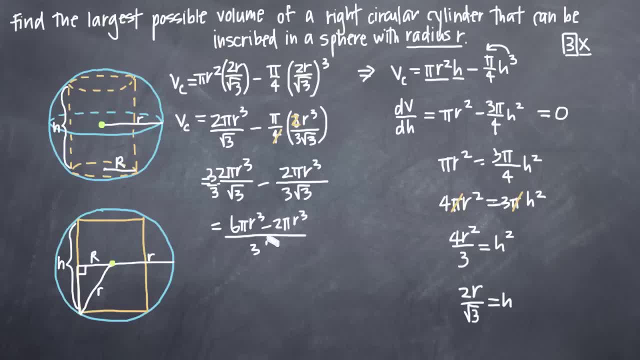 All divided by three root three. Obviously, that just gives us four pi? r cubed over three root three, and that's it. That's actually the largest possible volume of the right circular cylinder that can be inscribed in the sphere with radius r. 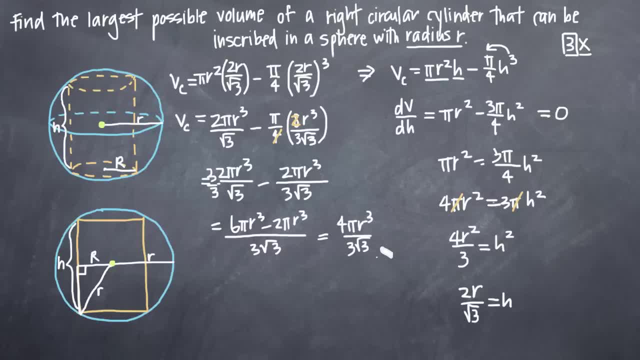 Now that we have this equation, what it would allow us to do is immediately find the largest possible volume of the cylinder, Regardless of the diameter of the cylinder, Regardless of the radius r that we're given. So, for example, if we were told that the radius of the sphere would be equal to two,